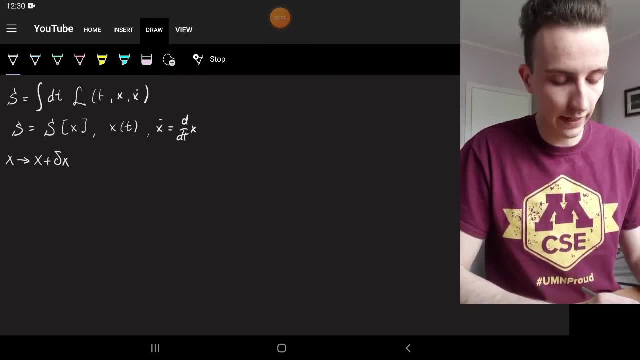 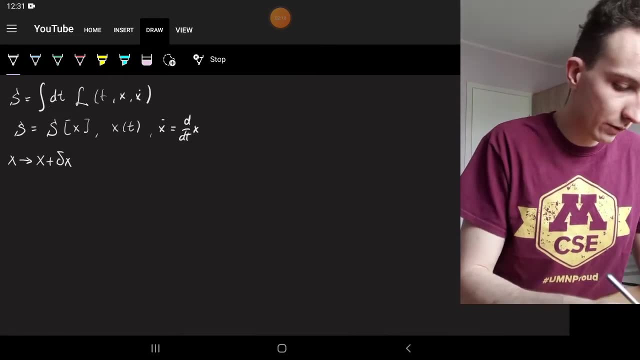 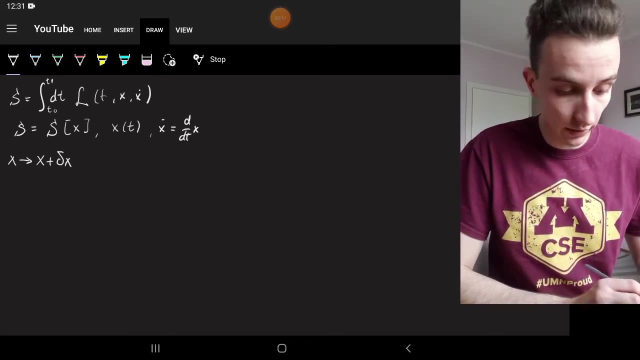 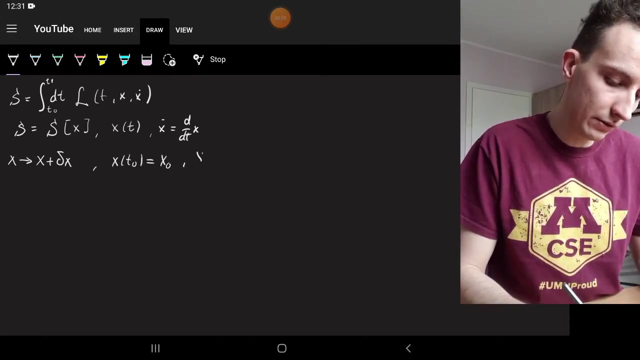 x plus delta x. x minus x x goes to x plus delta x. Now it's also important to note this integral. this integral is on an interval from t zero to t one. and we say that we know x of t 0,, it's x 0, and we say that we know x of t 1, it's x 1.. So this means: 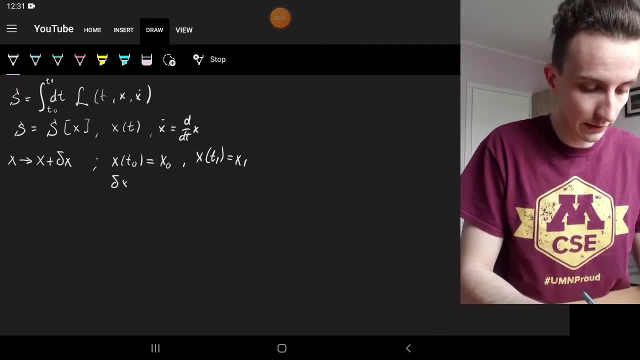 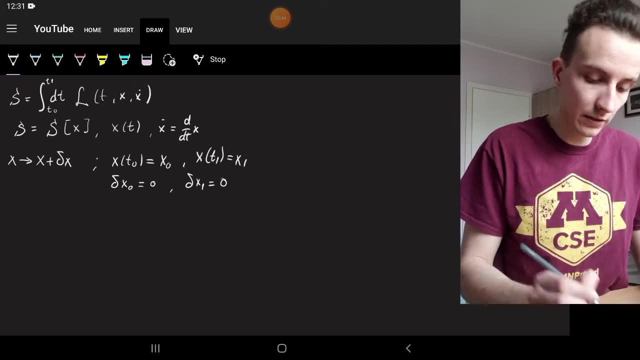 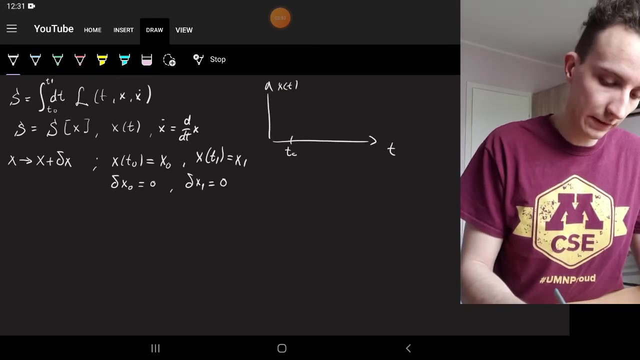 that in these points there will be no variation. So in these points delta x 0 is 0 and delta x 1 is 0. So this function x of t- let's say that this is t 1, t 0 and t 1,- this function could. 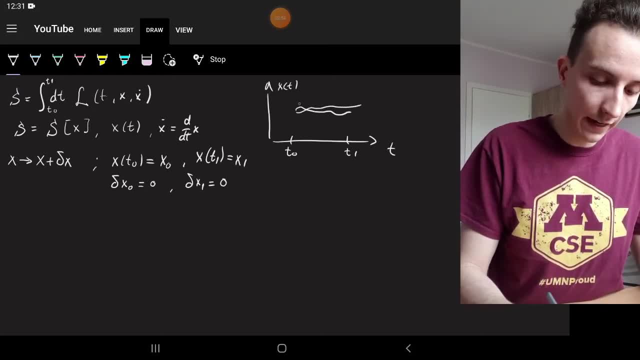 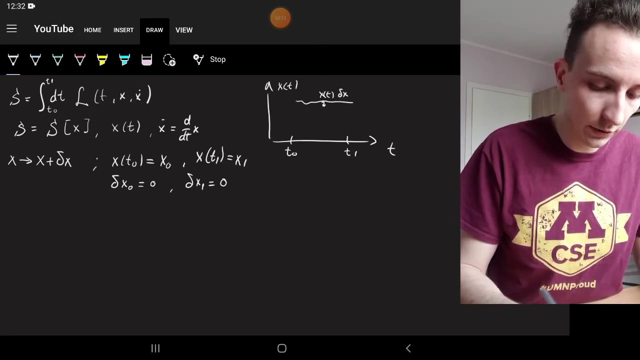 be. this could be that anything. Now, if it was something like this, that would be x of t, and then all of these differences would be delta x. I mean x of t plus delta x or minus delta x. But what's important to note is that they have to start and end in the same point. That's what 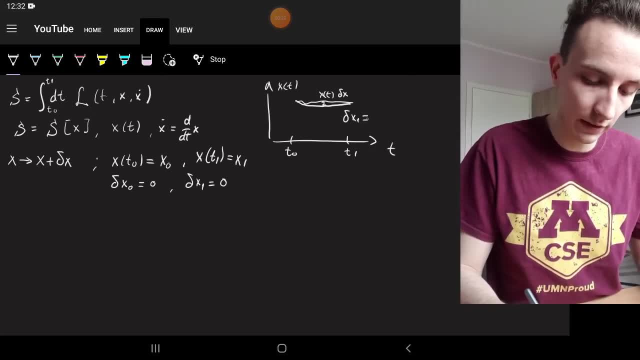 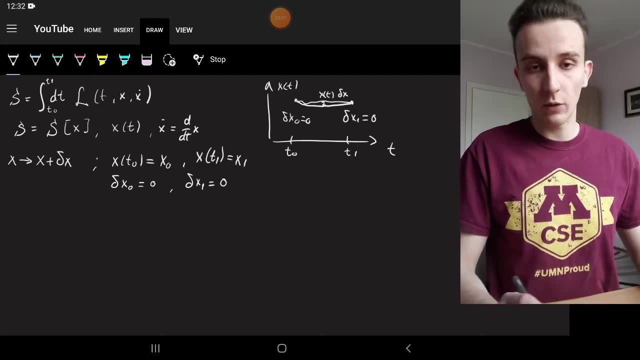 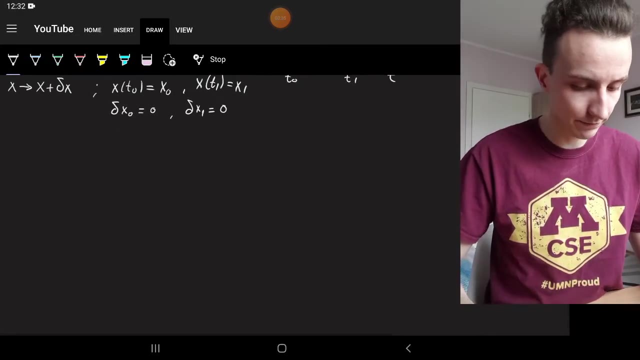 we specified by saying that delta x 1 is 0 and delta x 0 is 0. That's why they have to end in the same point. And now we're looking for which kind of these functions minimizes the action s. So we define this variation of s to be: 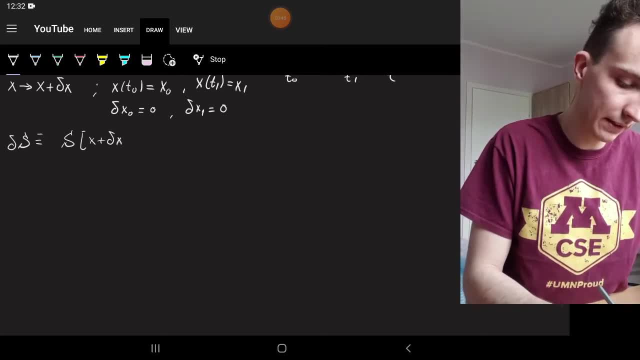 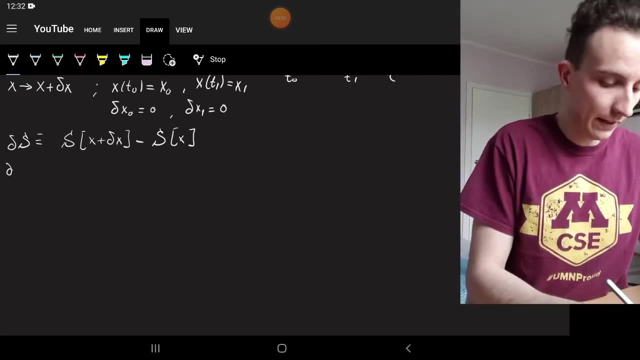 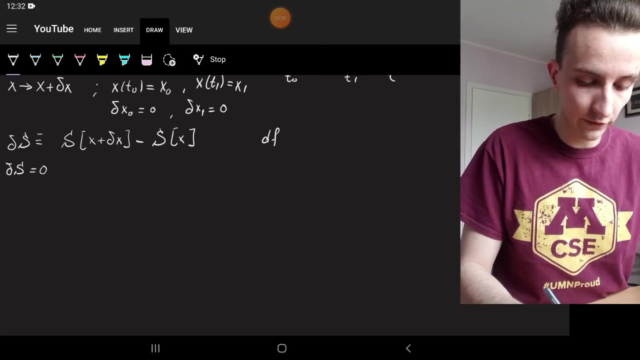 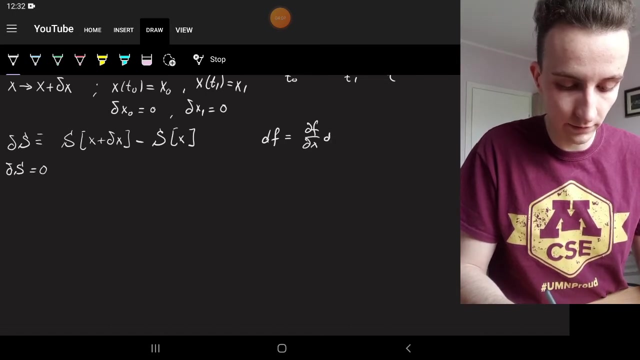 s of x plus delta x minus, just s of x, right? This is very much like the derivative. And then if we were to say that delta s has to be 0, you might recall that if you had a function of x and y and it would be like del f by del x dx plus del f by del y dy, And you were looking for 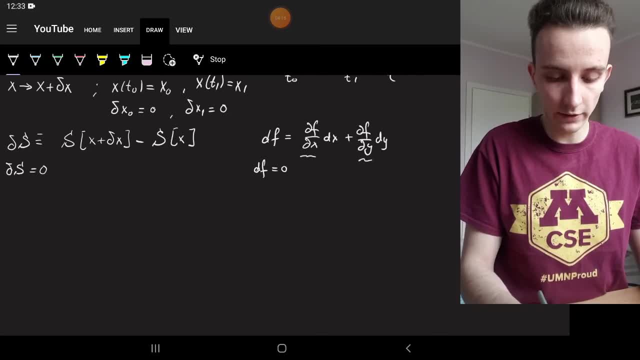 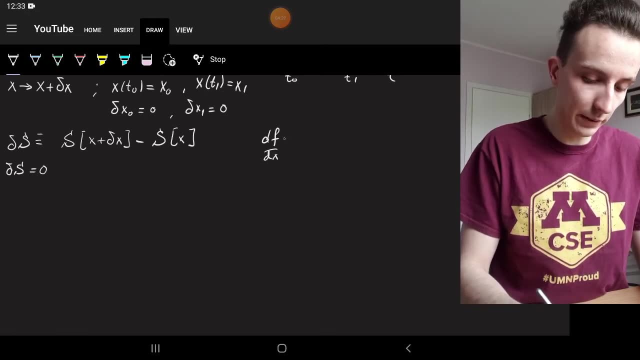 a constant f, And that would mean that all these partials have to be equal to zero, And, conversely, if it was just a function of one variable, that df by dx would have to be zero, right, which is the same as saying: 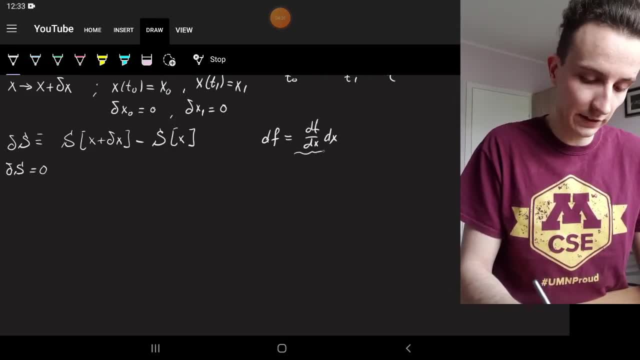 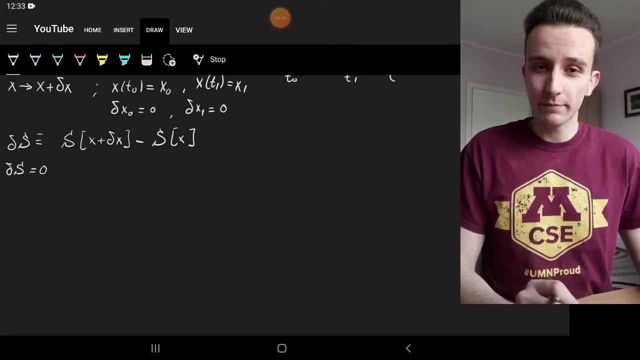 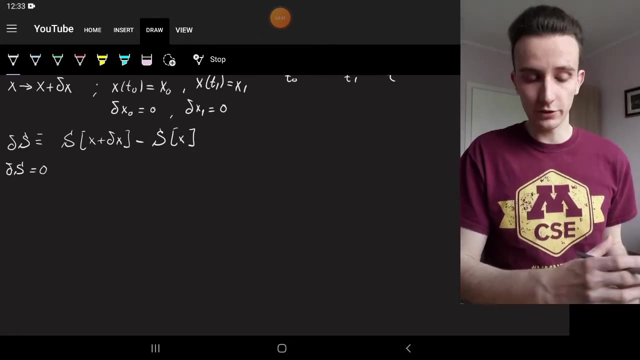 df by dx, dx. That's why- and df by dx is zero. It's gonna be the same parts with these variations. So we're going to be keeping only the linear terms of delta x to variation with respect to, and we're going to set its coefficient to be equal to zero in exactly the same analogous way. 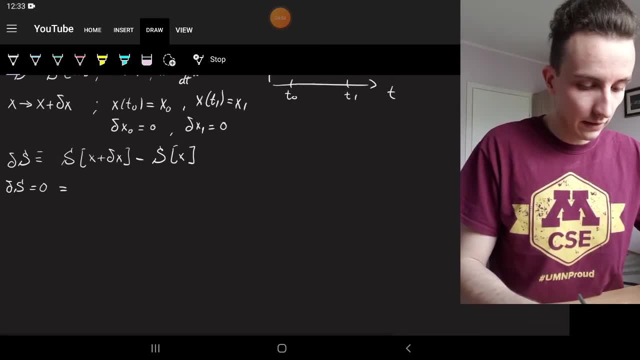 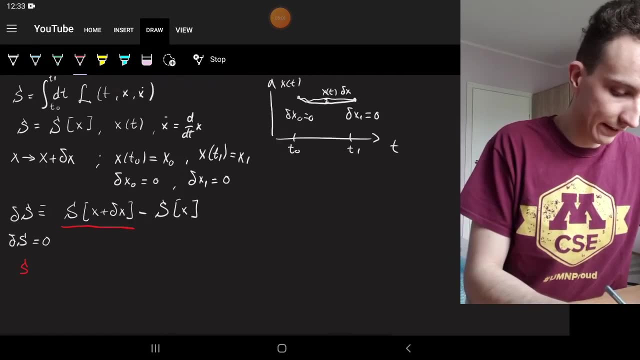 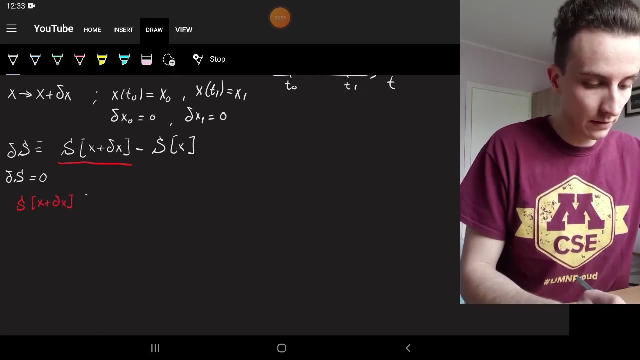 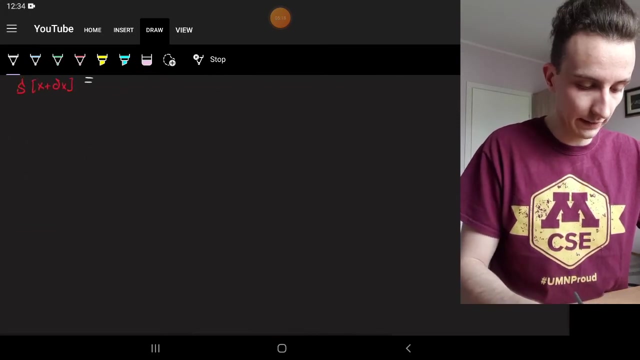 So now we're going to look at what delta S is. We might do well to first find this quantity. Here we go, I'll underline that, and let's find that. So S of X plus delta X is equal to- we're looking at this guy over here, when we add the delta X to the X's. 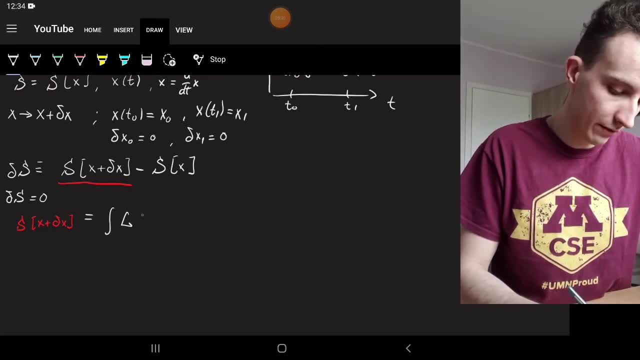 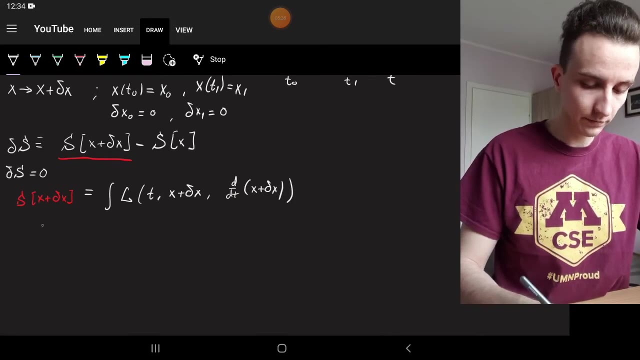 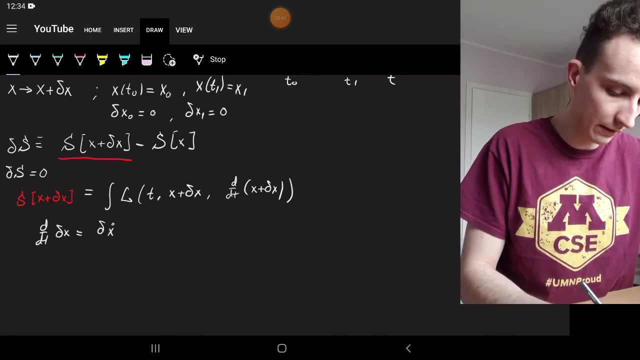 sorry, that's equal to the Lagrangian of T X plus delta X, and then this is D by DT of X plus delta X. Now it's good to note that D by DT of delta X is just delta of X dot. 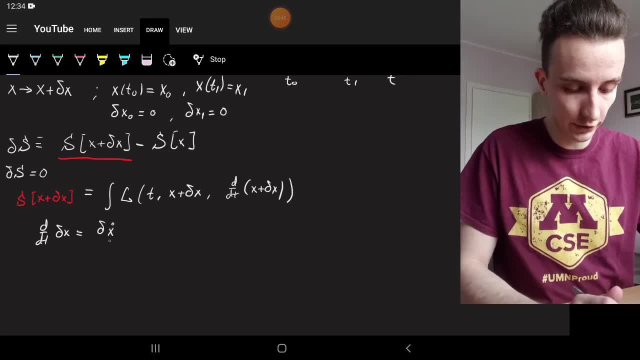 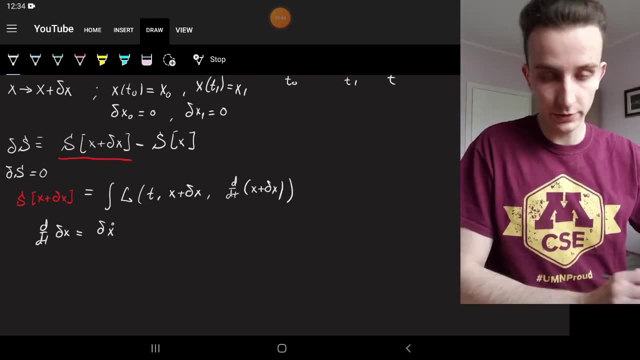 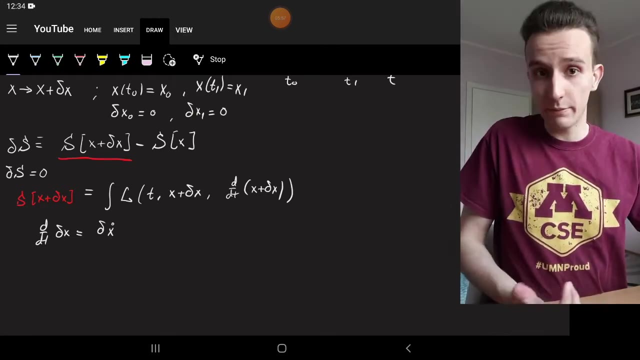 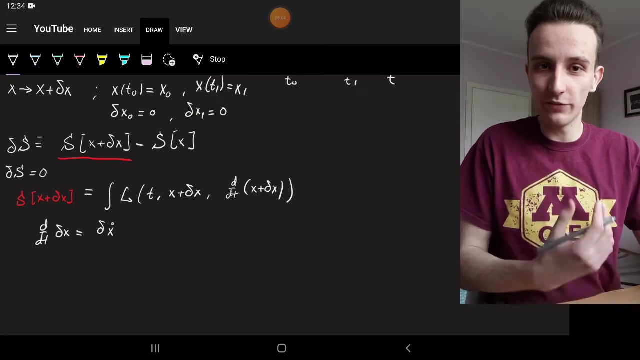 So they commute, the derivative operator and the variation operator commute. This is because, in our case, the independent variable, which is, in this case time, is completely known to us. It's absolute right. So we know it's at each point of time. we know the time, so there is nothing to be varied there. 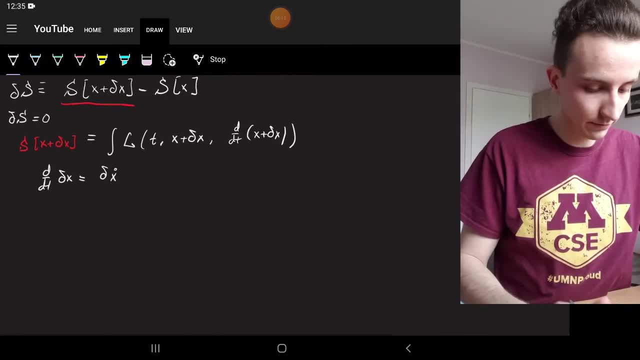 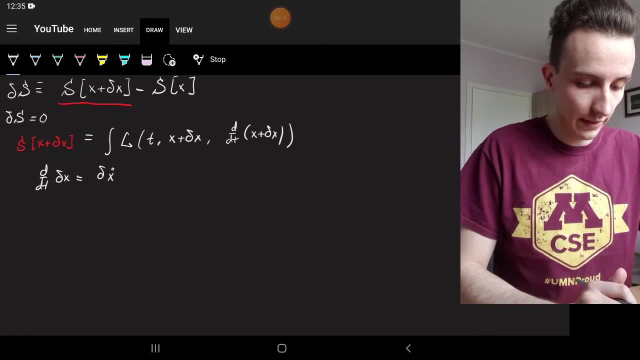 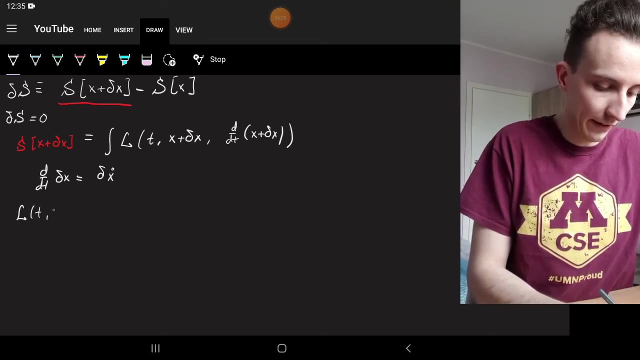 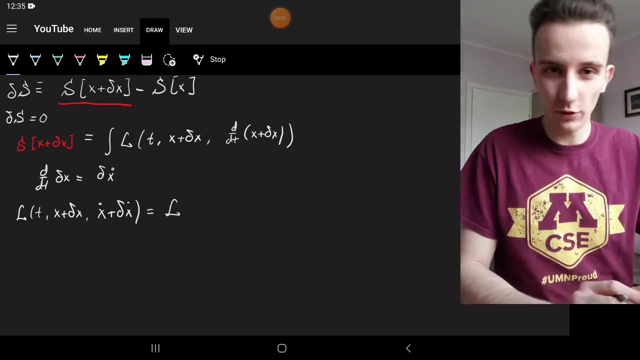 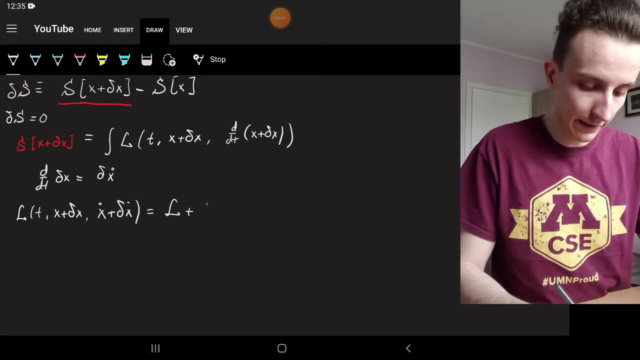 It's certain. so the time can commute with variation. Okay, so we have this, and now we need to Taylor expand this Lagrangian so that we would have linear orders of delta. Okay, I'm just rewriting it, And so that's going to be just our regular L of T, X, X, dot, plus this guy when I Taylor expand him. 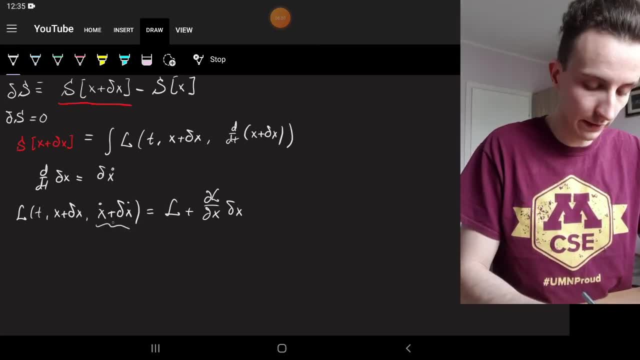 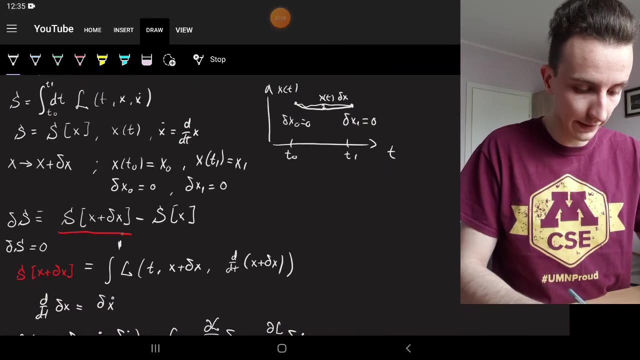 is del L by del X, delta X. and then, when I expand with respect to this, I get del L by del X, dot, delta X, dot. Okay, Okay. So now I'm going to be putting that inside here, and because the integrals are additive, we can put everything in the same integral. 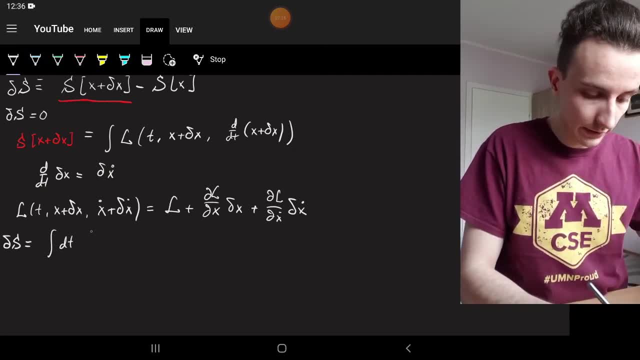 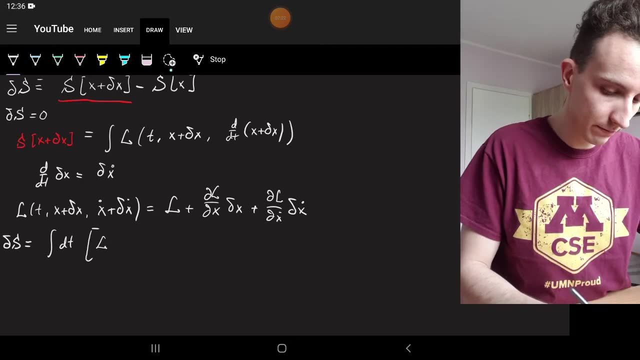 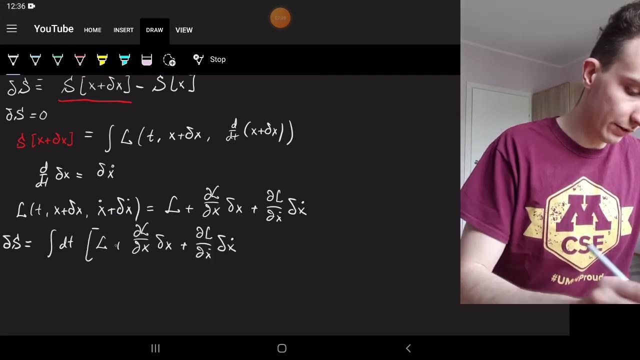 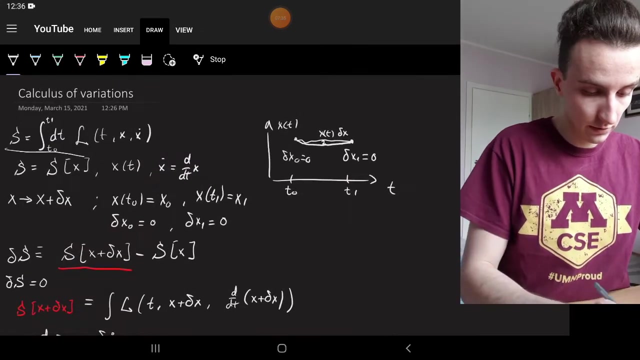 So delta S is going to be the integral DT. We have to. we put this part in. so we have the Lagrangian. let me just copy all that. We have the Lagrangian, its partial derivatives, Times the variation, and then we subtract the Lagrangian from this one because we said minus S, right. 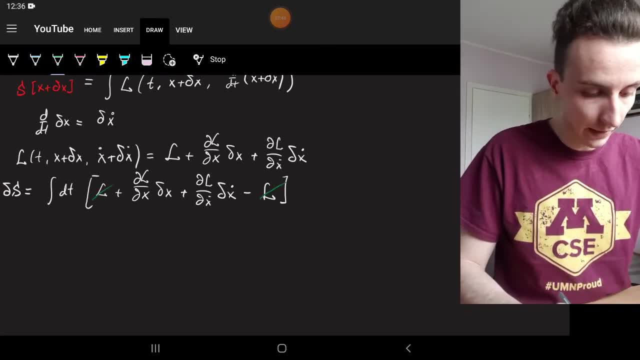 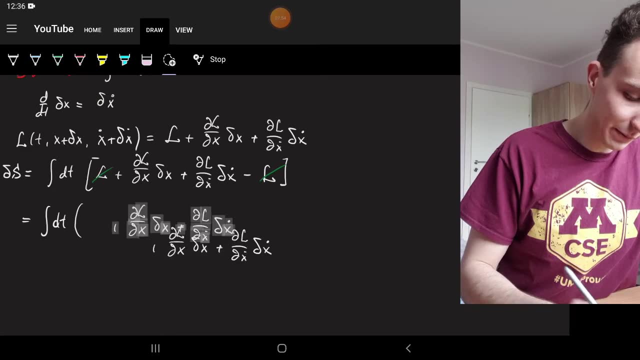 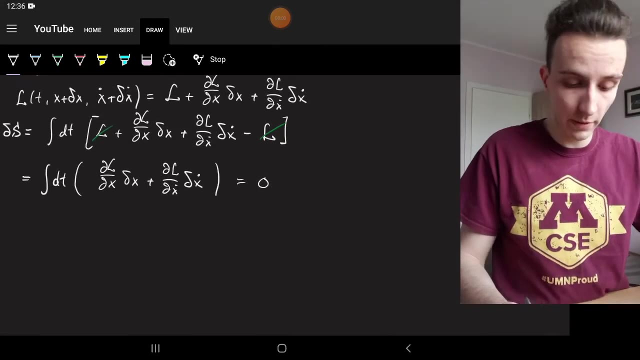 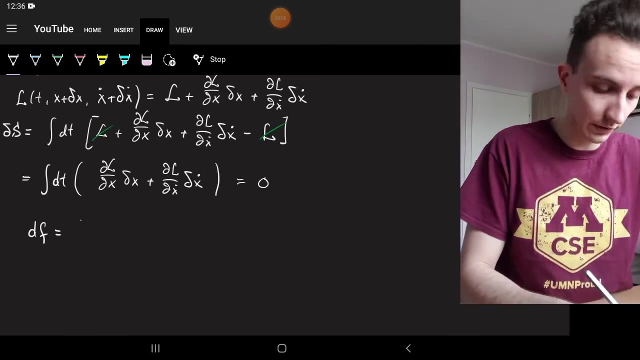 So these two guys will just disappear and we're left with DT, And luckily I have this copied right. That worked out just fine and that's supposed to be zero. Now remember what I said. like in the total derivative of a function of two variables, for example: 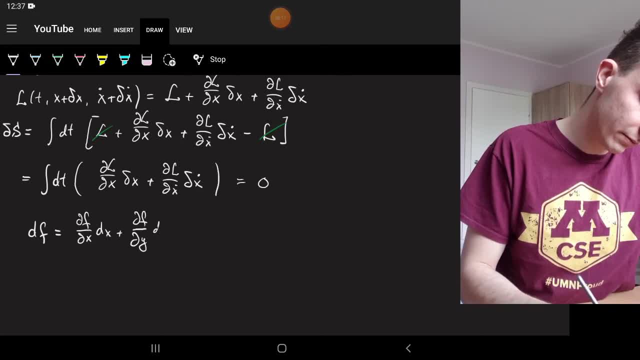 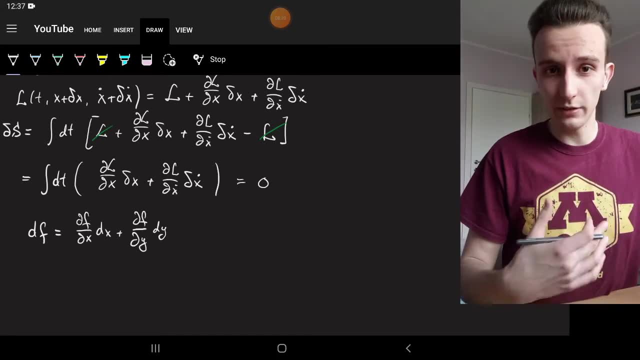 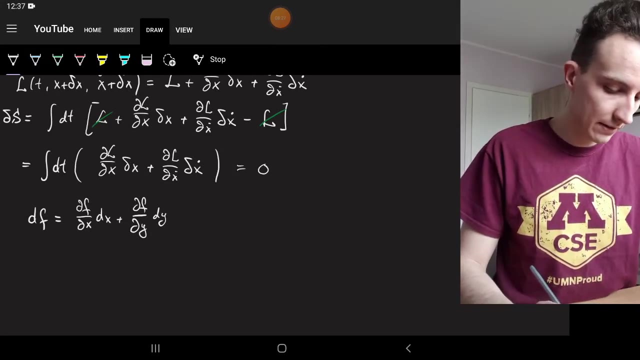 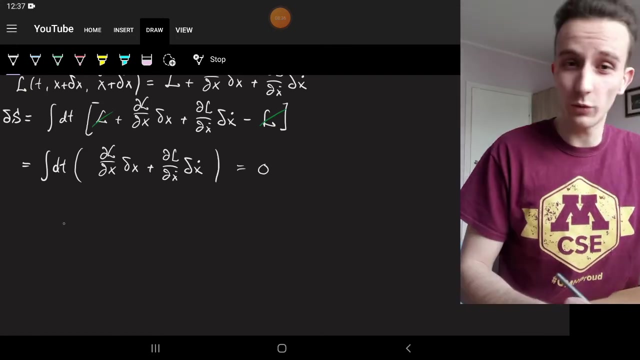 We want these to be equal to zero, But that's only if these DX and DY are mutually orthogonal or, you know, mutually independent. But delta X dot is definitely not independent of delta X, So we need to express it with respect to delta X before we can do any of this. shenanigans and equate coefficients to zero. 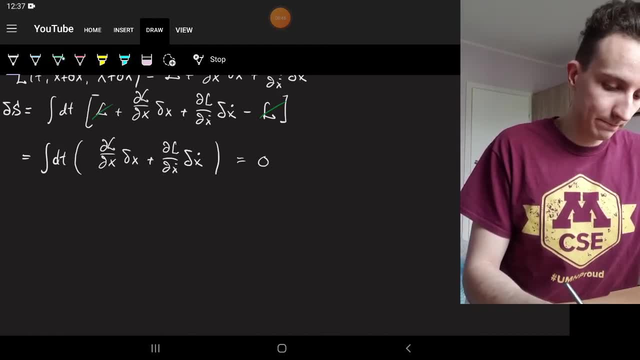 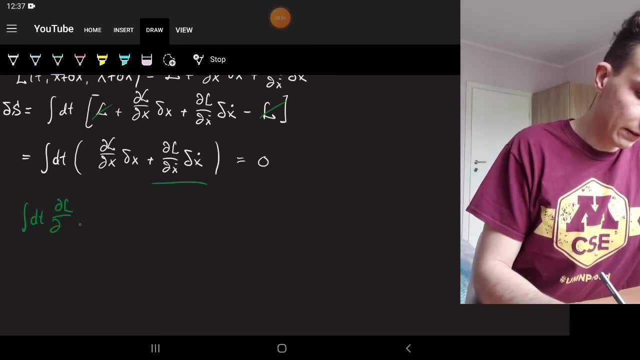 So we want to look at this term as we underline it, and I look at DT, delta L by delta X dot, delta X dot. I look at this one So we can note that, you know, this is a constant right. 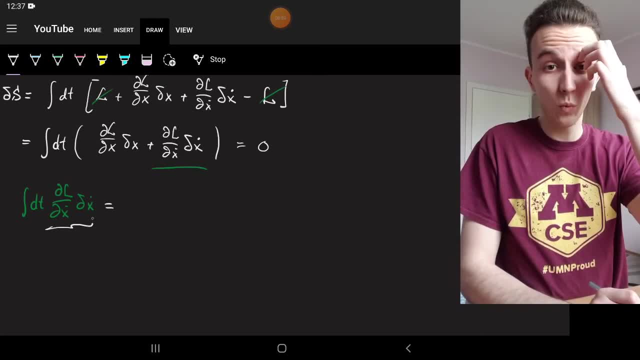 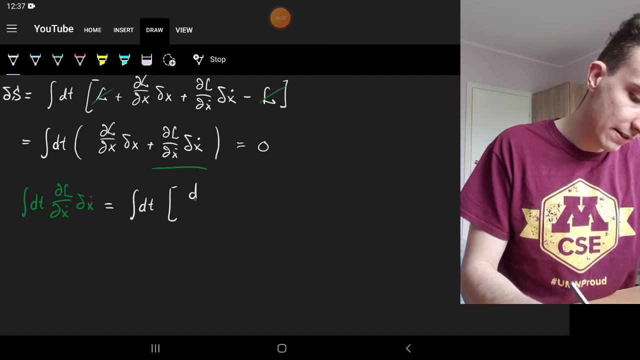 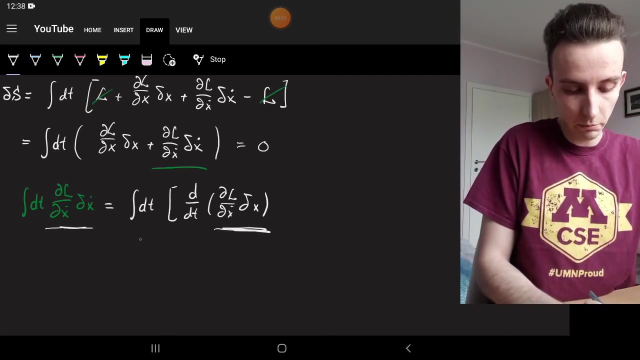 We can notice that this is one of the two results of a product differentiation. So I can write this as DT and then D by DT of delta, L by delta X, dot delta X. So if we look at this, if I differentiate this part, I'm going to get this plus another term. 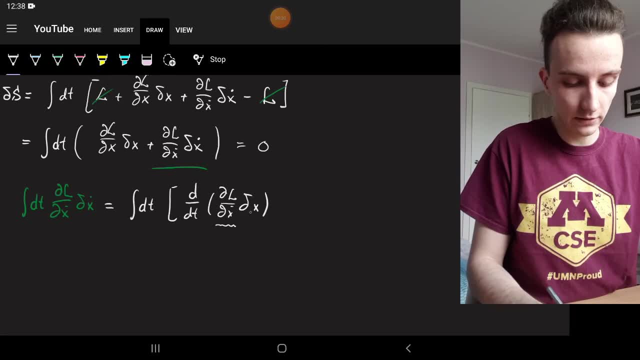 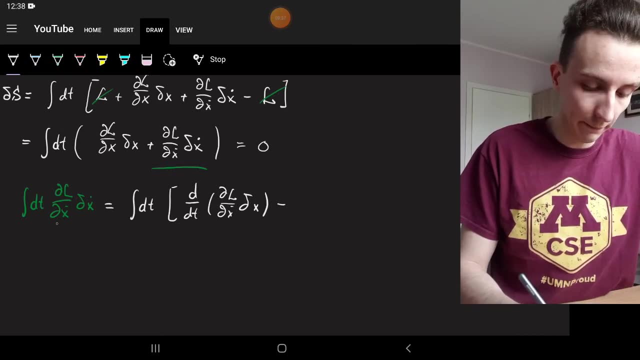 This guy differentiated With respect to time plus. I mean time is just this other function, right? So I have to subtract that away because I just have this in the left-hand side. So on the right-hand side I have that. 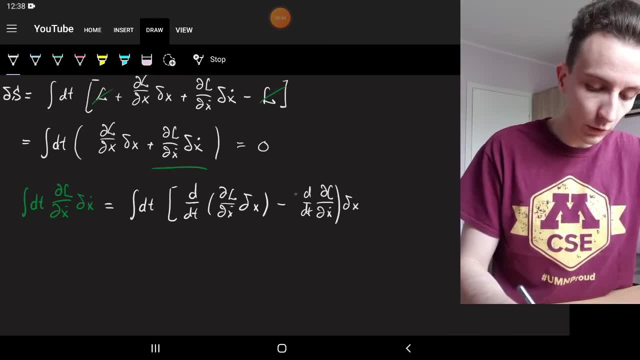 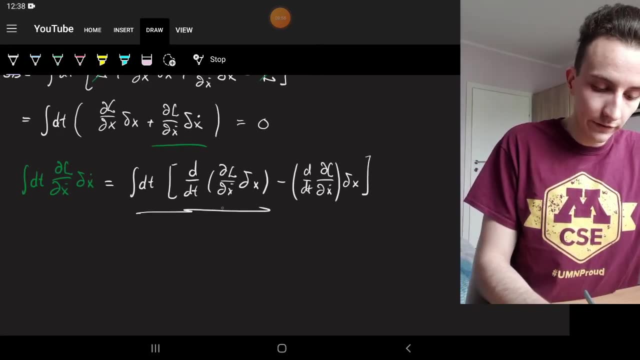 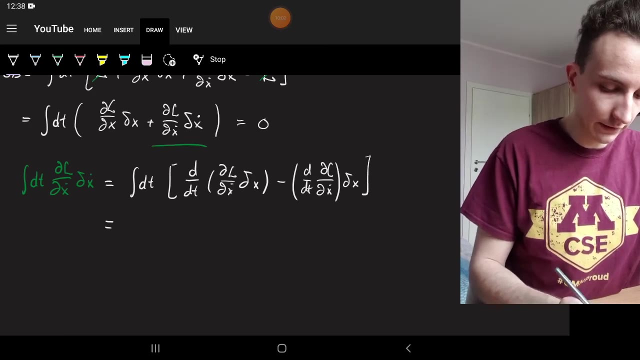 This plus- I mean minus- this, where only this is differentiated now, And what's really nice is that we can get rid of this term. We integrate it out. So this whole thing is: oh yeah, there's no integral for the first one. 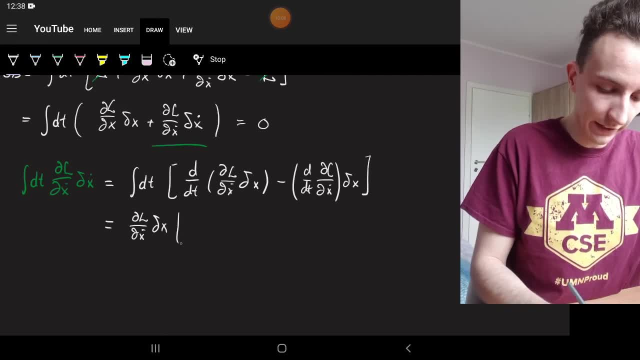 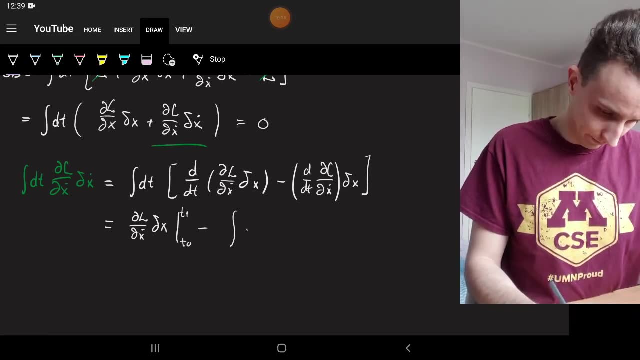 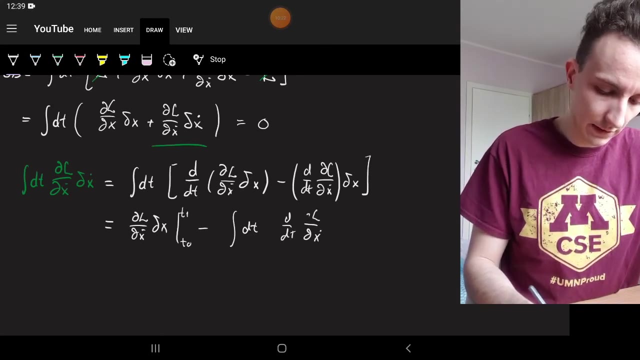 We integrate it out, like I said, delta X, And it's evaluated on the boundary, So that's D0, T1 in this case, minus the integral DT D by DT of delta L, delta X, dot. God, I hate writing partials. 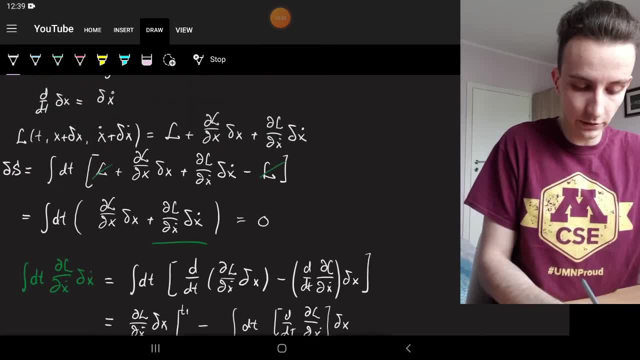 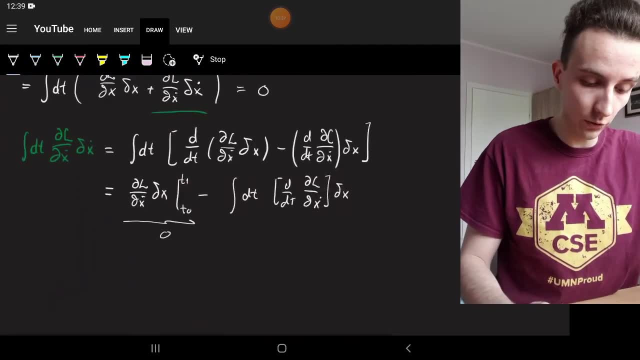 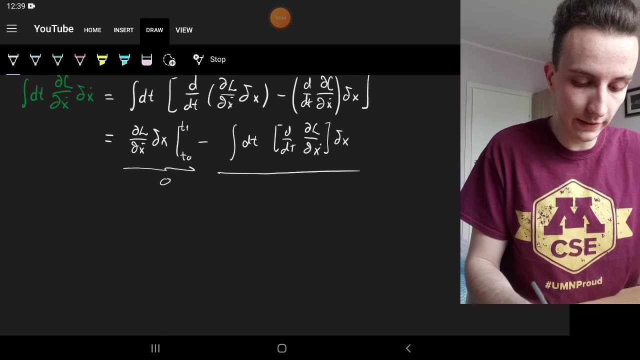 Delta X And this part goes to zero because, like I said, the variations are equal to zero. And the boundaries? we know what the value of X is at the boundaries. Okay, So we keep only this term, We keep only that term and we put it back in. 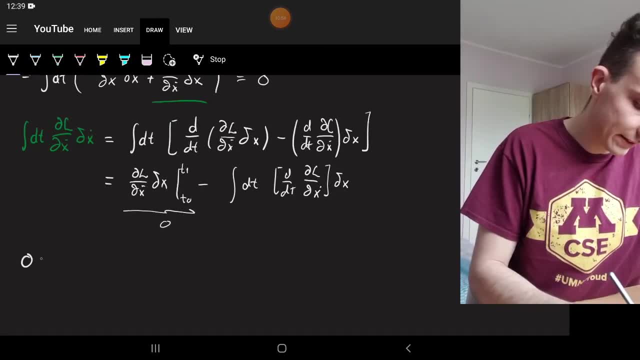 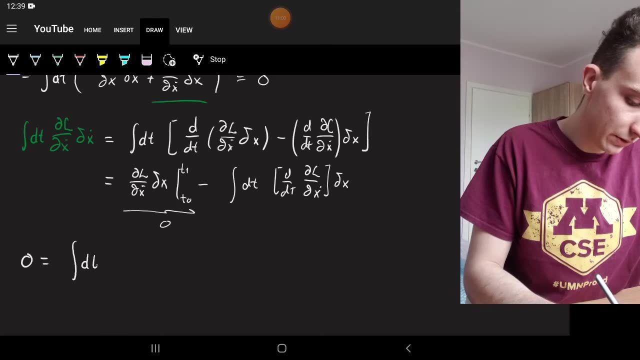 Now we've got everything with respect to delta X. So we have the zero, which is the variation of S, is equal to well, which is what we want it to be equal to, is equal to the integral del sub T. 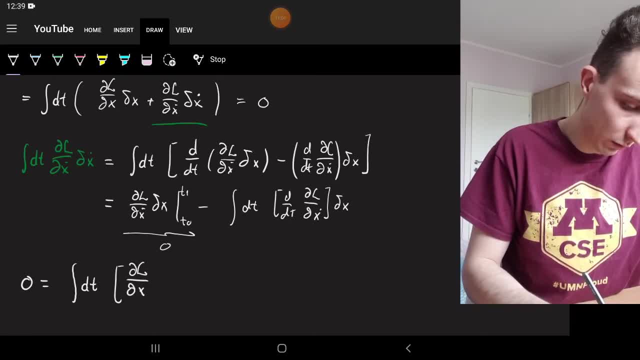 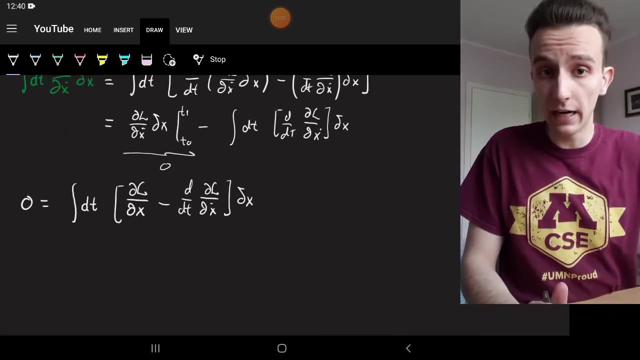 We copy the first term, So that's partial L, partial X. I'm going to put delta X in front and then minus D by DT. partial L, partial X, dot, And then I have delta X, And now we can set this equal to zero. 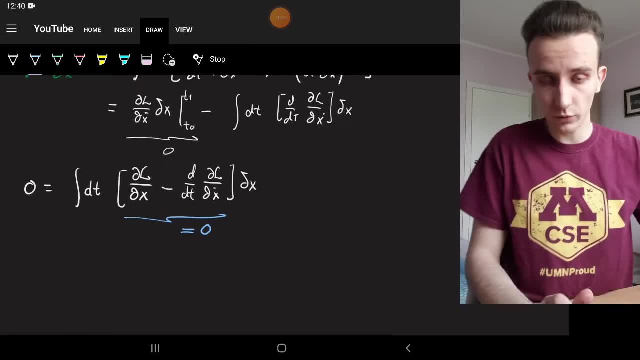 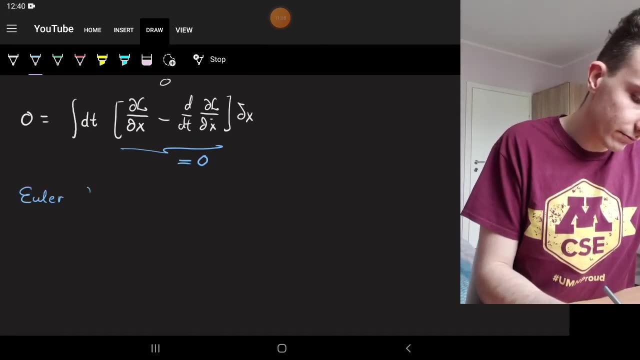 Because it's the only way that this integral is always. it's the only way that this integral is always equal to zero, regardless of delta X. So if that's equal to zero, then we get the Euler-Lagrange equation. Euler-Lagrange equation.